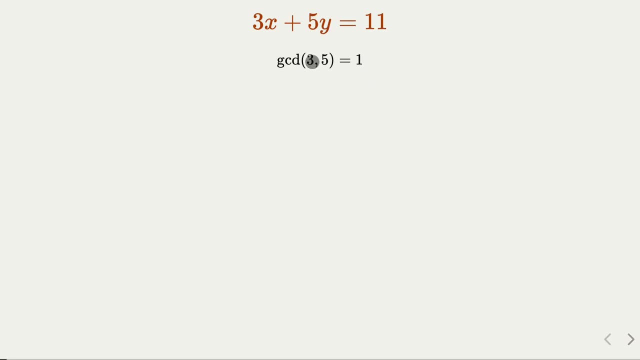 and 11 is not a multiple of 3.. On the other hand, if this 3 and 5 is a co-prime, then we have infinite many solutions. How to find a particular solution? We use what is called extended Euclidean algorithm. 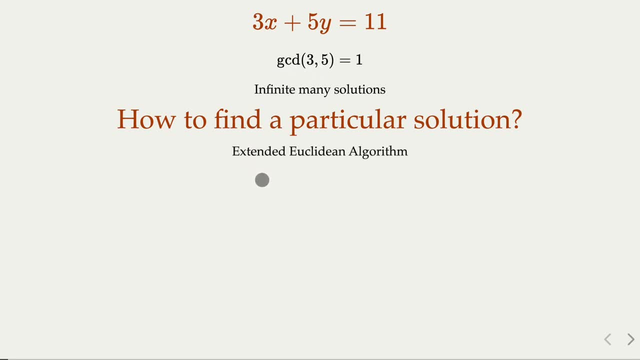 and to find the gcd. In this case it's trivial. you know a negative 2 and 1, that would be a particular solution here, right, And in this case because we have 11, so we multiply by this by 11,. 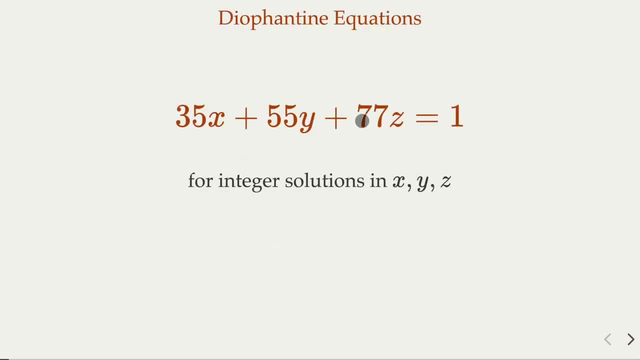 that would be a particular solution. And let's go back to our problem. with three variables, Introduce three different methods. In the first method, we're going to split this into two equations. How do we do that? So look at this equation. here We can rearrange it. 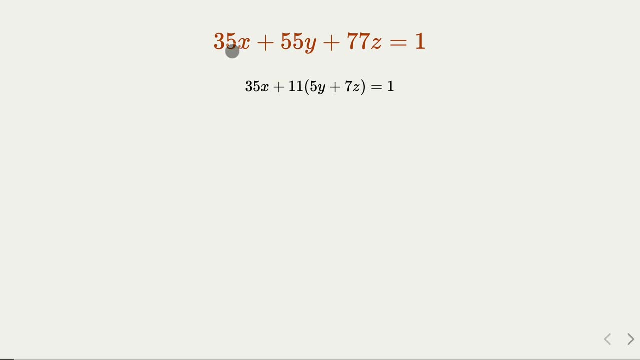 This is a common factor. 11: here Notice that the three numbers are co-prime, so this has infinite many solutions And we're going to say this is going to be an integer here. so let's put this into two equations, where this is the integer w. 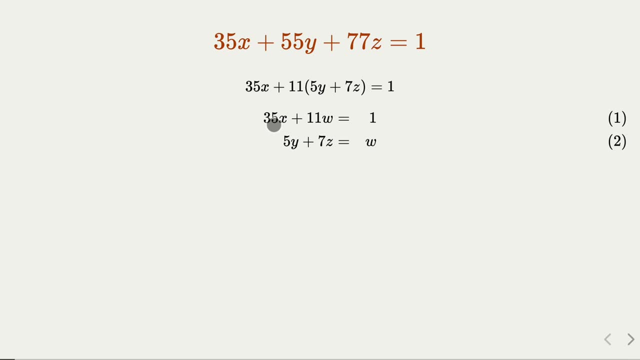 for this term here, And the original equation becomes 35x plus 11w, equal to 1, and 5y plus 7z, equal to w. Now notice that these two equations both have solutions. Why? Because the gcd of the coefficient is 1 here. Okay, so how do we find the solutions Now? we can just solve. 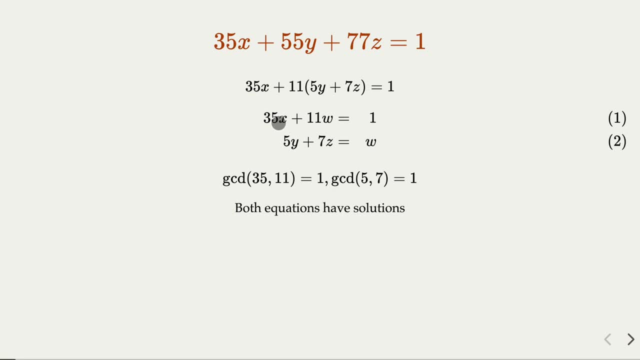 the equation by using this equation here. Now we can just solve the equation by using this equation here By using the method we described earlier, because each has two variables, right. So let's do that. Let's start with the second equation here: 5y plus 7z. 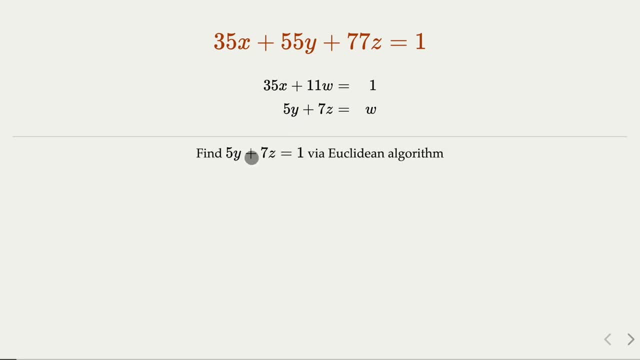 Let's start with w equal to 1.. How to solve this equation? Now? we're going to find a particular solution. You're creating an algorithm here. We're going to skip the steps. but three and negative two is a particular solution. So general solution from earlier result is going to be D. 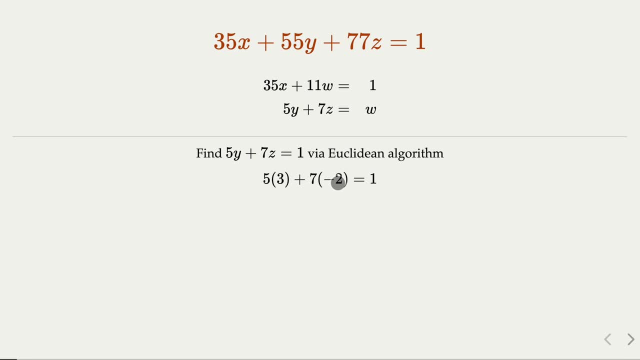 So the general solution from earlier result is going to be D, this one. Of course, this is the equation for equal to one, But we're looking for w, so we multiply w in order to satisfy the new equation here. So y and z in terms of s, s, 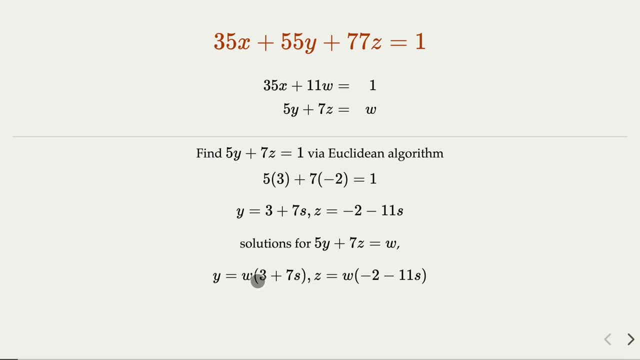 is the integer and w. So what is w? W is the solution for the first equation. So let's go back to solve the first equation here, that is 35.. We need to find this. the gcd here right is one. So use Euclidean algorithm. we find that it's negative. 5 and 16, alright. 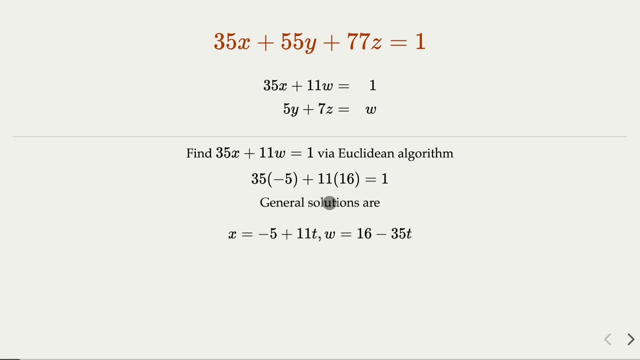 So with that, a particular solution is found, and general solution is going to be like that. So we solve x and we solve w in terms of t. Now t is in the integer here. Come back and find the two results. what do we get? We're going to get you know for these two. 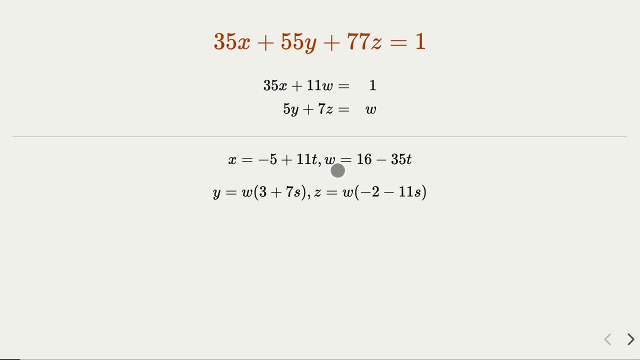 equations. here we know that for the first one we have this solution, and here everything can be expressed in terms of s and t. So we have two parameters, and then we have an intermediate value of w, and then x, y can be expressed in s and t or w, which, of course, in return 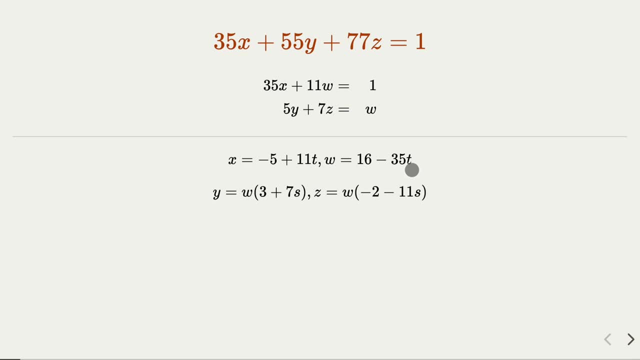 can be expressed in terms of t. okay, So the solution here is x, y and t. So the solution here is x, y, z, yeah, and where s, t are parameters. That's the solution. That's the first method, that is, to split into two linear differential equations with: 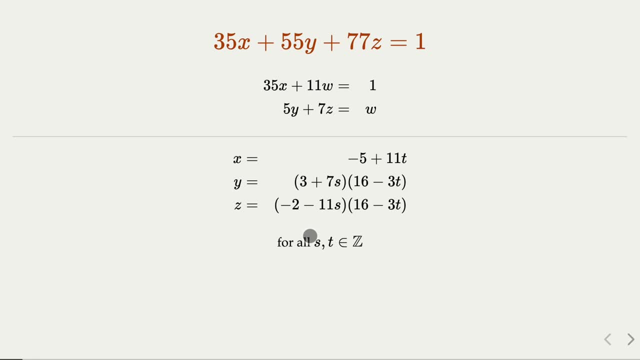 two unknowns and then combine the result at the end. alright, So give example, you want s t equal to zero, then this is going to be a solution here. you can verify that, okay, Alright, so this is one class of methods. 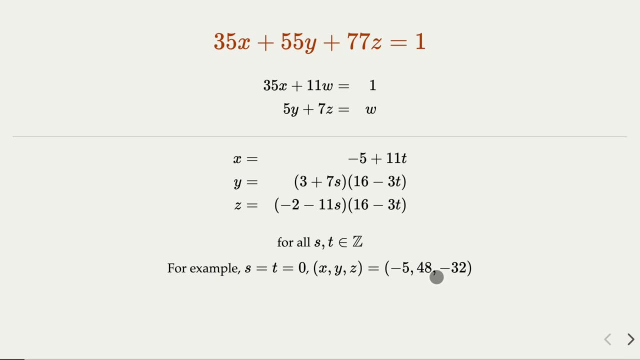 You know, in solving multiple variables. let's look at the second method. In this method we try to use parameter with what is called a canonical form. So what do we mean by that? So notice that for this equation, if there's one coefficient here- that is one- then the 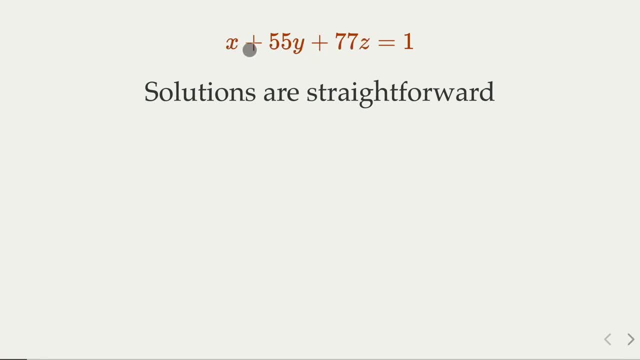 solution is straightforward, right, even though we have three variables in this case, since this is an intermediate value, Okay, If there's one here, of course, the gcd is always one, always has infinitely many solutions. and how do we find the solution? 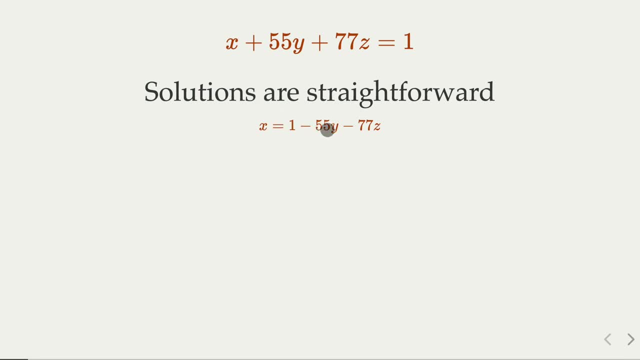 It's straightforward: just express x in terms of y and z, where here y and z can take any integer values, and then this would satisfy the equation, and the solution is straightforward. So that's good, but of course in our case it's not even close. this is 35, there's no. 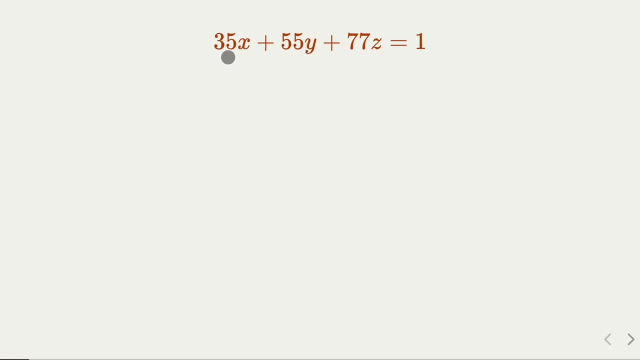 one here in the coefficient. So how shall we do that? It turns out that we can move toward that, so we're going to choose the coefficient here with smallest absolute value- in this case it's going to be 35, and we're going to express: 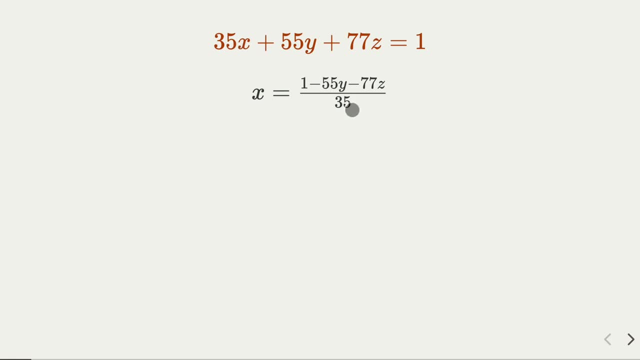 x in terms of other values here, and notice that you can do some algebra here, because this is 55, you can split that into 35 and 20, this is going to be 70 and 7.. So let's work out the steps, all right. 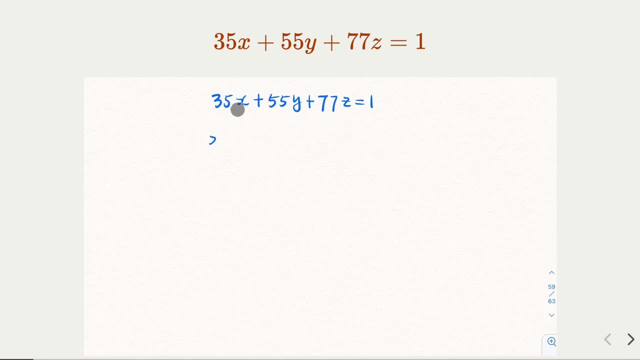 So here we start with the original equation. we choose 35, the smallest, and then we express x in terms of the fraction here: 1 minus 55y, minus 77z over 35.. And then for 55 and 77, we're going to keep the integer part, and that is, we have the 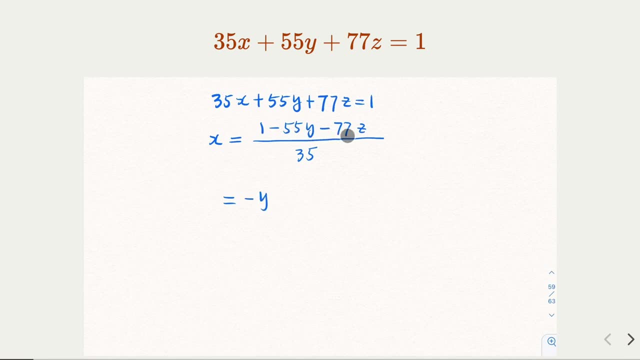 one negative y and negative 2z, minus y minus 2z, and then the fraction still remains, that is, 1 minus 20y minus 7z over 35.. Of course we're dealing with integer solutions, which means this whole fraction must be an. 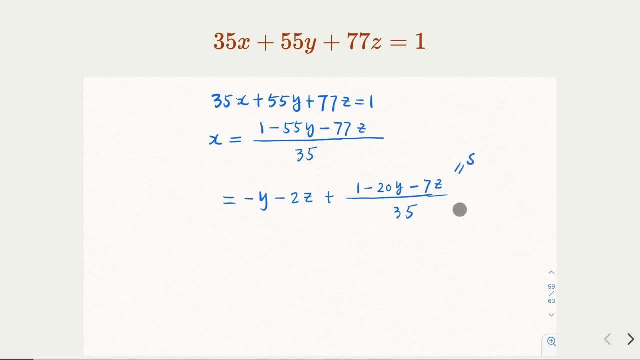 integer. Let this integer be s integer s right. So what that means is: s is an integer and, of course, in this case, x you can express in terms of y, z and a variable s. And what is s? 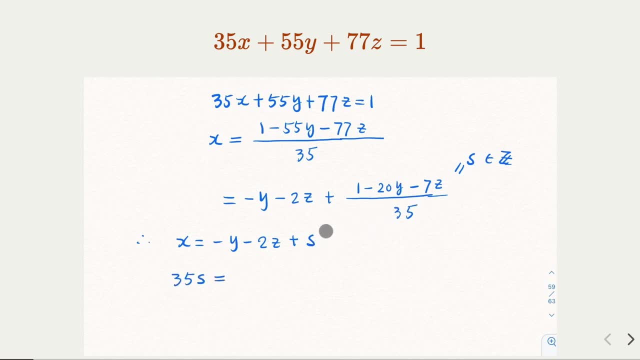 s is this fraction here, which means 35s, would equal to 1 minus 20y minus 7z. Now here we turn the original equation into a new one, New variable: s we get rid of x, right. 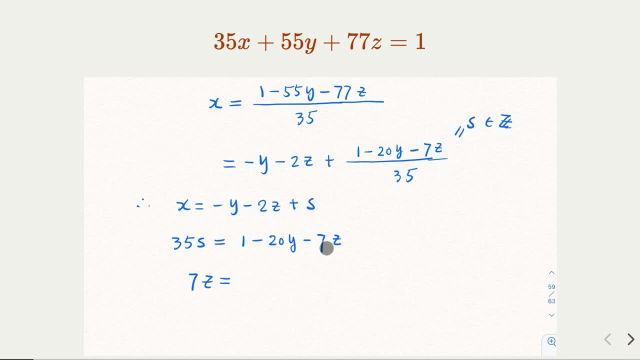 Now, here we work with smallest absolute value, which is 7,. so 7z equal 1 minus 20y minus 35s. And then z to the fraction here. okay, is the whole expression here divided by 7.. 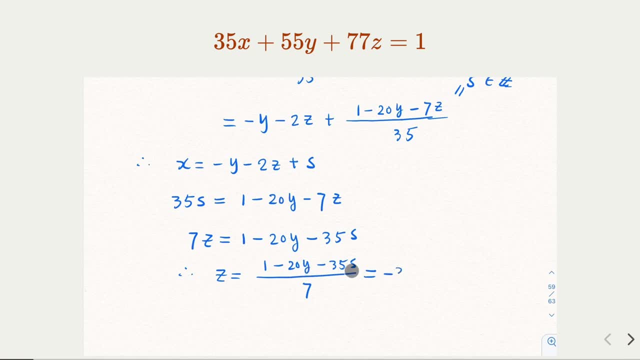 And of course, we're going to take the integer part of y and s here. right, This would be 7z. Okay, So we're going to take the integer part of y that's negative, 20y maybe, and then plus. 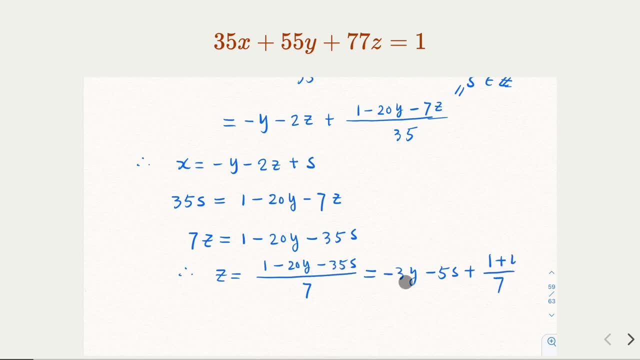 y. This would be multiple of 7, that's good. So negative: 3y minus 5s plus 1 plus y over 7.. This must be an integer. Let's call it t right? Integer t. t is an integer here. 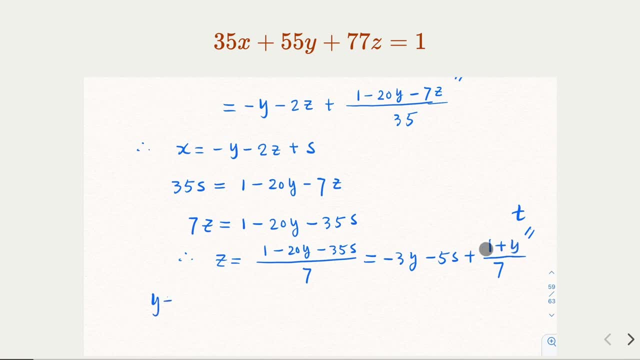 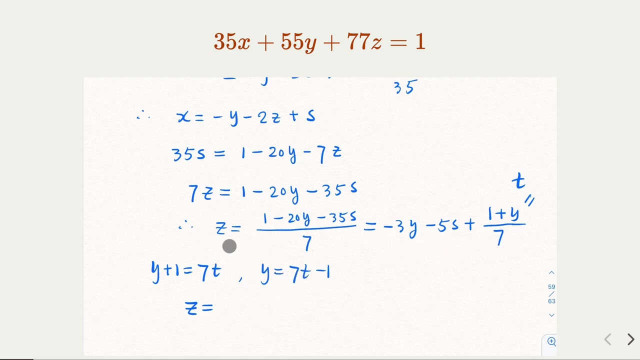 So in that case, y plus 1 would equal 17,, and then y would equal 17 minus 1.. Okay, Notice that now we expressed Okay. Notice that now we expressed 17 minus 1.. Okay, So we're going to plug in y in terms of t. 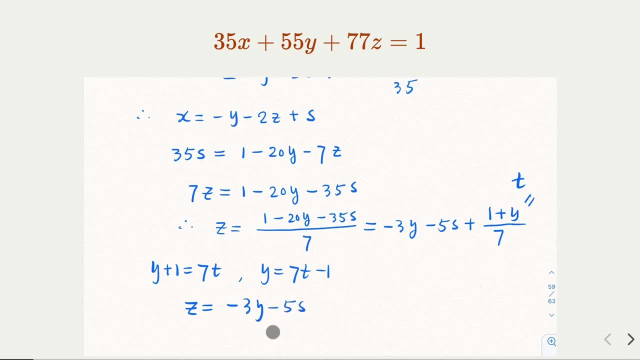 But z here just plug in here is going to be negative 3y minus 5s and plus t. Now you notice that we can pretty much express everything in terms of either s and t here, right. So here, what do we have? is we're going to plug in y here, right? 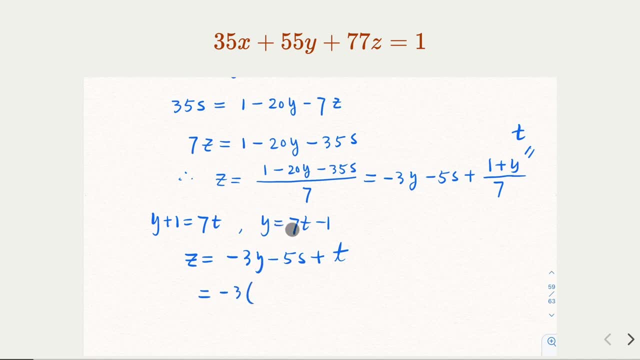 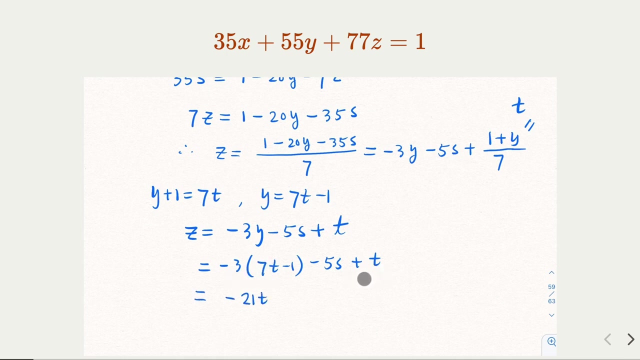 17 minus 1 here We're going to plug in y here, right, 17 minus 1 here In this expression here: So minus 5s plus t, and then we're going to combine the term here Negative 21 plus t, that's negative 20.. 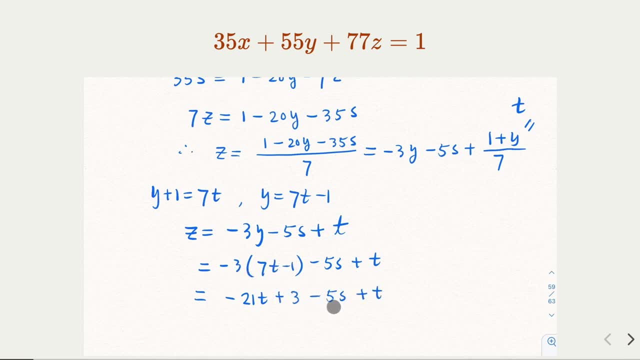 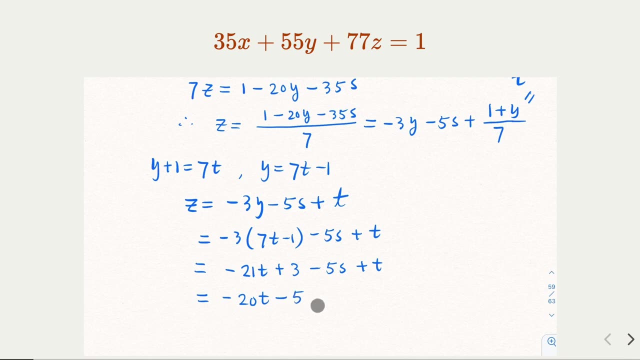 And then this minus 3 becomes plus 3 here Minus 5s, So further combine the term Negative 20t minus negative 5s plus 3.. Alright, that's good. Now we express z in terms of s and t. 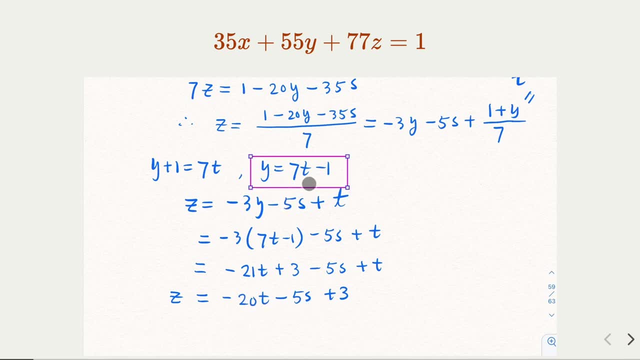 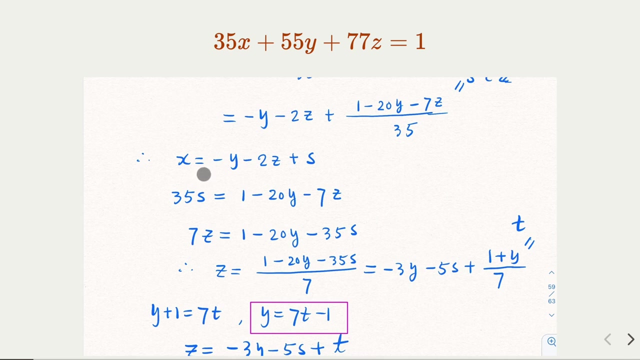 Alright, We express y in terms of t- Yeah, And z in terms of s and t. Okay, And we express the Originally. we have x, right, So x is also Now here. we have y and z, So we need to replace y and z with s and t. 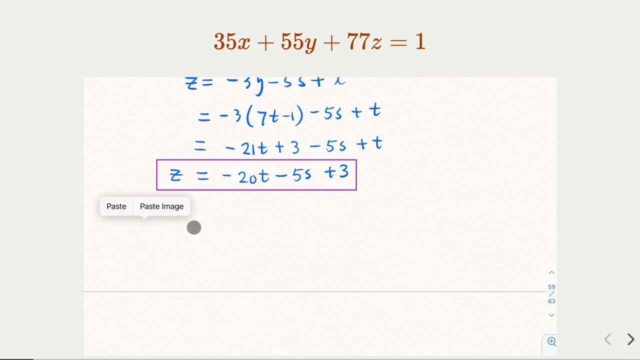 Let's do the algebra here, Alright. Let's copy it over here, Alright. So that's x in terms of yz, And we want to get rid of y and z, right? So just plug in the y value here, which is 17 minus 1,, right. 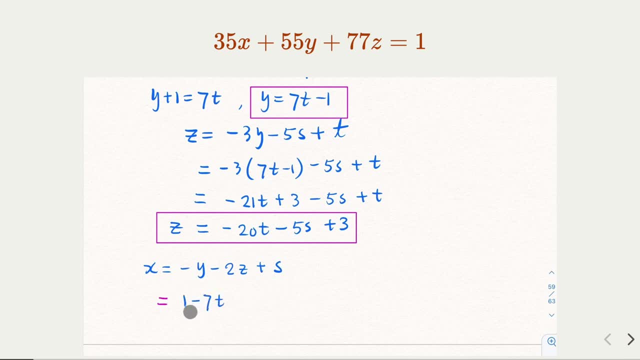 So plug in here, Flip the sign 1 minus 17.. Minus 2z, Minus 2.. Times z, This whole expression. here we just plug in: Yeah, Like 20t minus 5s And plus 3.. 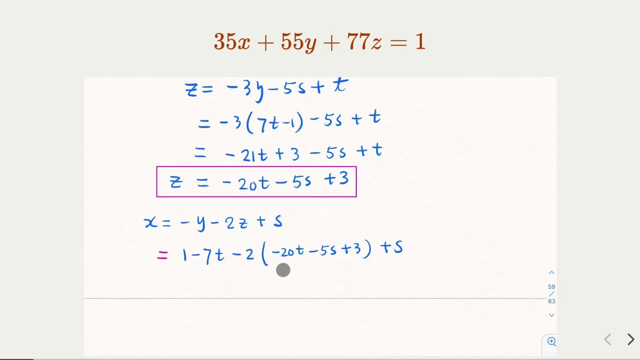 And then we add s. Now we're going to combine the terms here, right, So that becomes 1 minus 17.. This is going to be plus 40t. Yeah, Because negative, negative, is going to be plus And plus 10s. 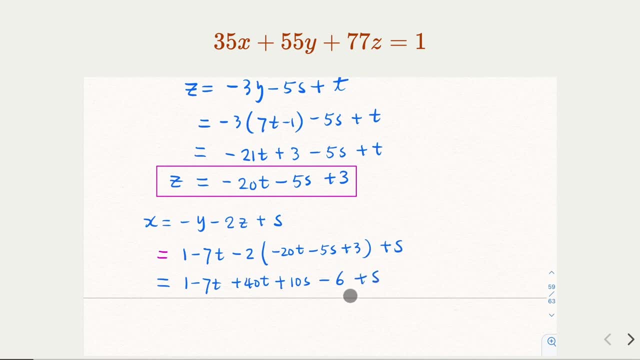 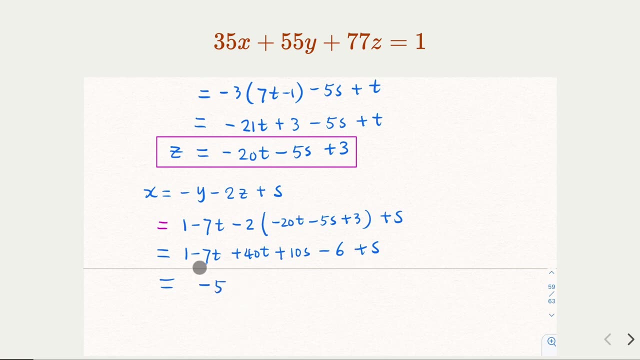 And minus 6. Plus s And further combine the term. What do we get is negative, 5. Constant term. And then we have 10 and 10. 10. 10. 10. 11. 11s. 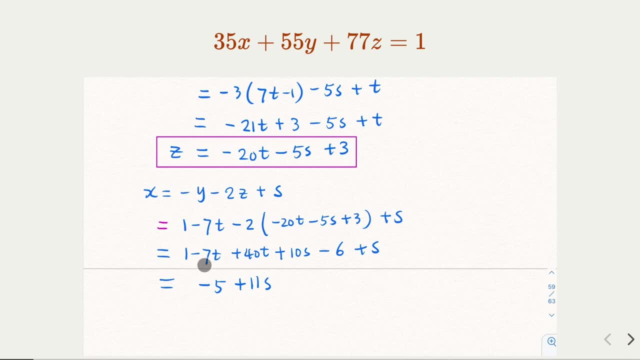 Yeah, And then for the t is 40 minus 7.. Yeah, So that would be 33.. Right, 33t. OK. So now we're done. Right, So we express everything in two parameters, s and t. 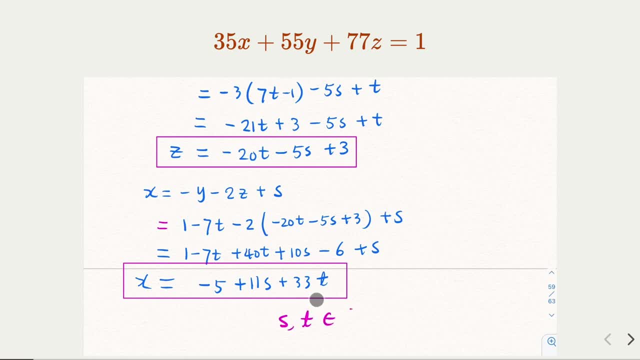 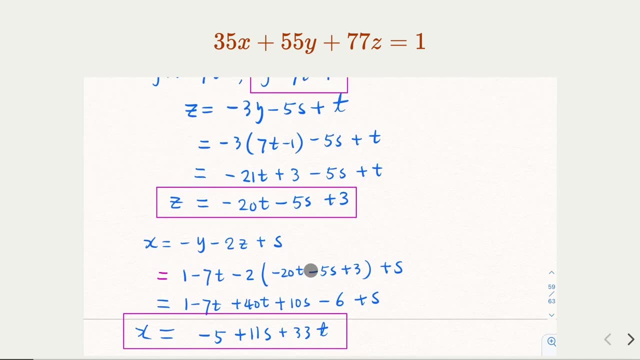 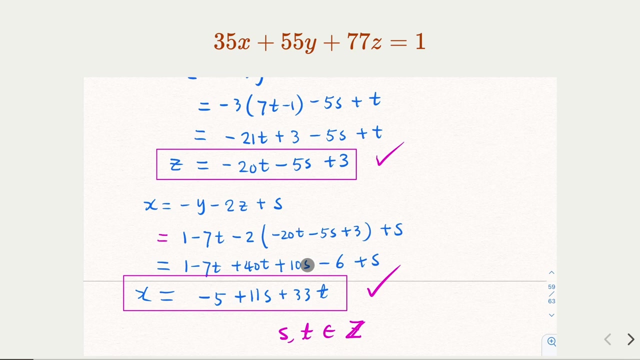 OK, Yeah, So that's good. So we solve the equation using this method, where we try to use parameters, and then we try to change the original equation by looking at the coefficient with smallest absolute value, And then, through three major steps, we're able to solve X, Y, Z. 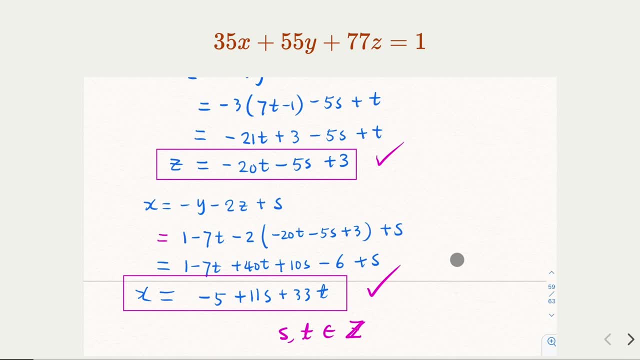 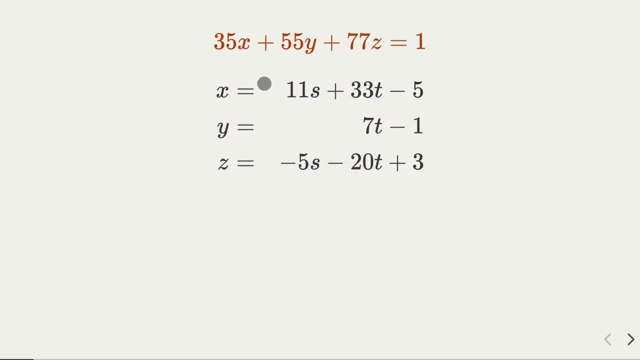 in terms of two parameters, S and T, where S and T can take any integers. So, in summary, that's the solution here. Look at that. This solution looks different from the original one, but both would cover all possible solutions. So let's move on with method number three. 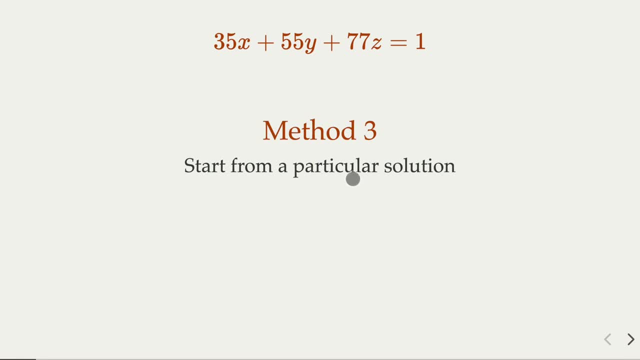 In the third method we're gonna start from a particular solution and then we're gonna use a generic solution by changing this constant to zero. Okay, So that is what do we do here. We find a particular solution that satisfies this X zero, Y zero, Z, lot here. 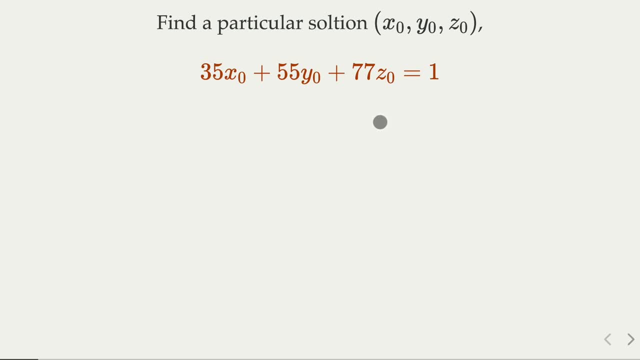 such as this original equation here: Once we find, once we have that, and then we're gonna find a general solution by changing this to zero. So imagine that if you do the summation X, zero plus X would be a general solution to the original equation here. 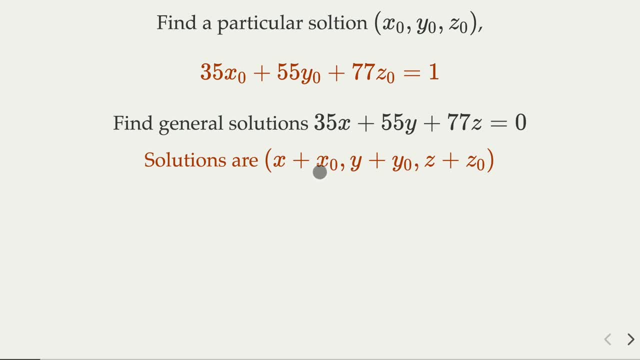 Right? So that's the step. So general solution is gonna be X plus this particular solution, X zero, Y zero and Z lot here, Right? So let's try. let's try out: How do we find that particular solution here? 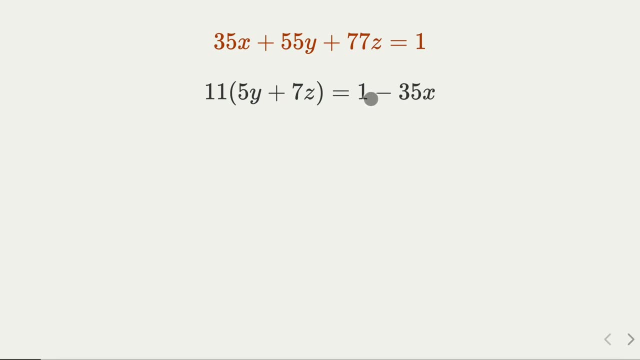 Okay, We're gonna rewrite it So you can just say: this has to be multiple of 11.. You're gonna try an error and X lot is gonna be six, for example, And the whole thing is gonna be 11 times negative nine. 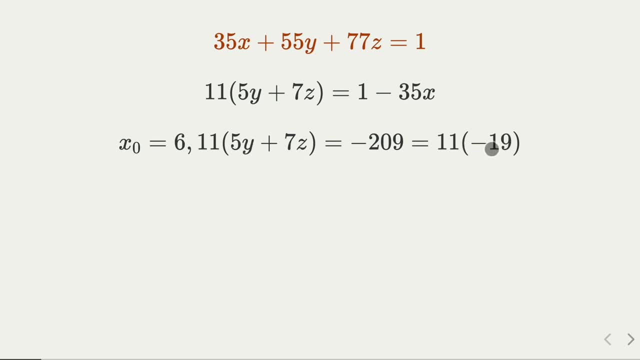 So that's gonna be negative 19.. So, which means five Y plus seven Z would equal negative 19,. right, And we try to find a particular solution. right, There's no burden to find a generic solution Now, that's easy, right. 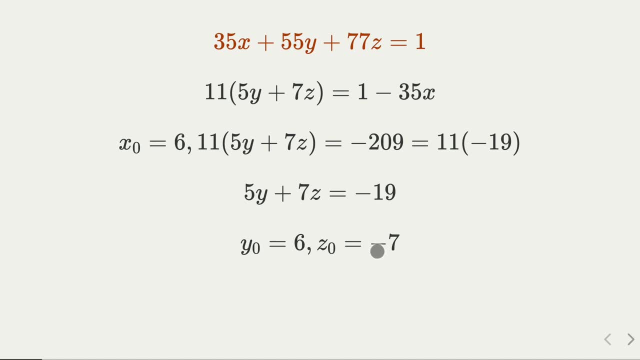 We can just let Y be six and Z be negative seven, That is, we have found a particular solution to this original equation. Now we're gonna find, as a next step, a general solution, a constant to zero right, Which makes much easier to solve. 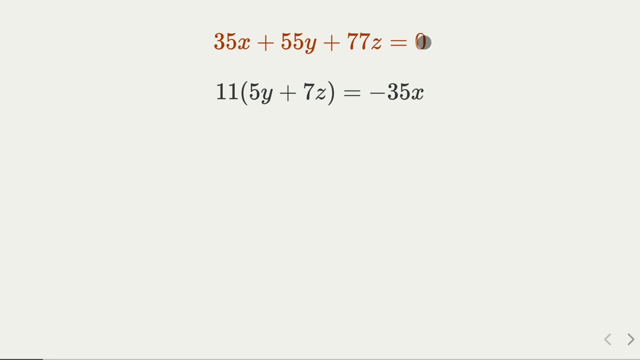 Okay, So change to zero. here I can combine the terms. Notice that X has, because this is 35 and 11 is core prime, which means X must be multiple of 11.. This X equal 11 S, right, Then plug in there, which means five Y plus seven Z. 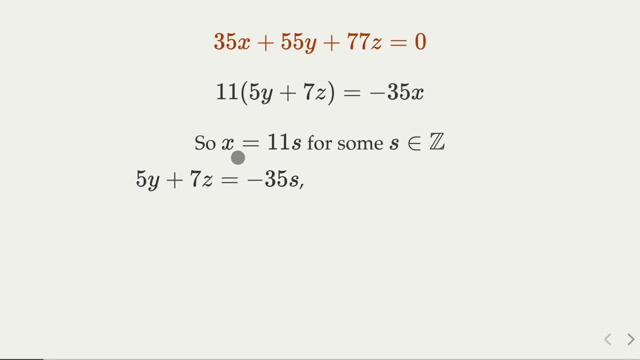 equal like 35 S, right? Just plug in This equation: X equal 11 S. Now, with that change it, So the five Y equal negative seven times some integer here Now, which means Y has been multiple of seven, right. 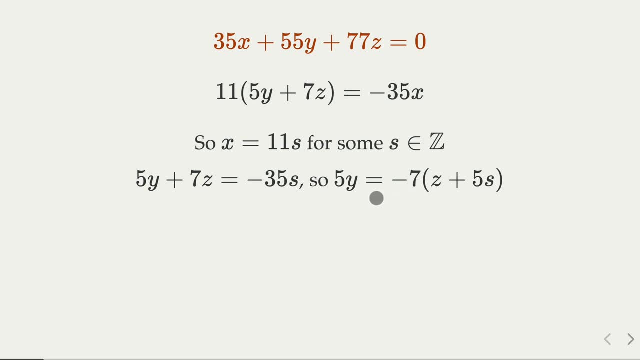 Because five and seven core prime. So which means we can say: Y equals seven, T or another parameter, right. So we have parameter S and T again. In this case you plug in and then Z is also zero. We can also express in S plus T. 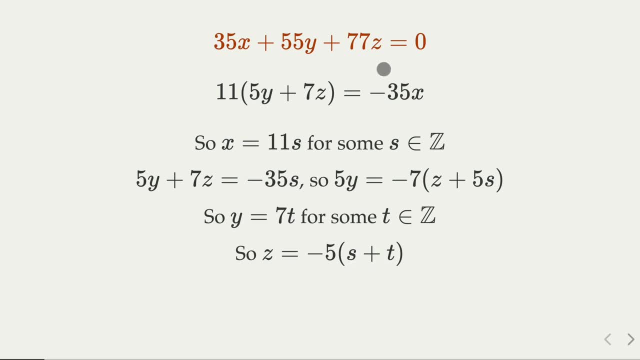 That is, we find a general solution, which is much easier because we don't have a. we don't have a constant here, We have zero here. So the solution here to this equation is gonna be with two parameter: S and T, that's gonna be X, Y and Z, right? 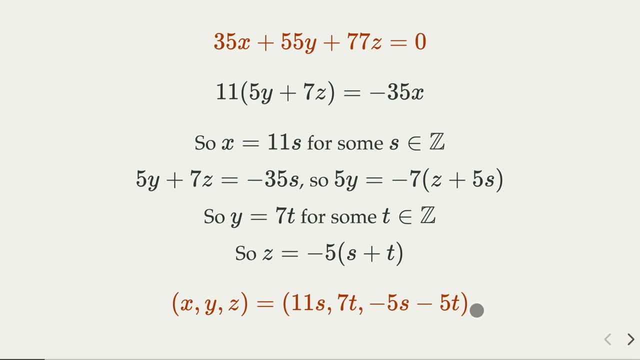 Now, earlier we said that what is the solution to the original Da Vinci equation? We can just do the summation of this general solution with parameter S and T and the particular solution right, This particular solution right, And this is general solution. 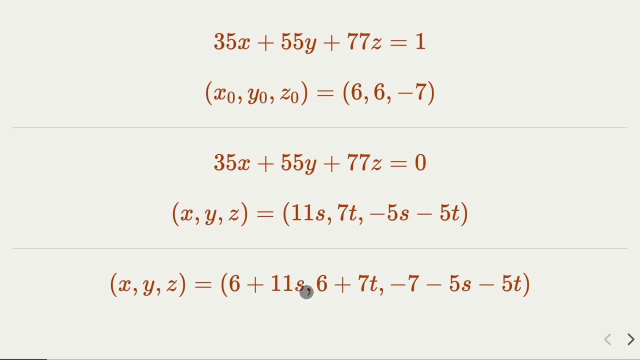 So overall solution is gonna be just, you know, summation of these two right And parameter is S and T. okay, So, in summary, we have used three different methods in solving the equation And notice that the method you know. 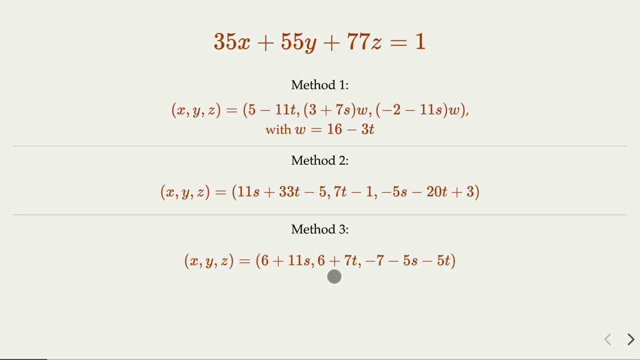 looks all different, right, But again, as I said, this is a different way of representing the numbers and you can try it out offline and they should cover. you know, you can prove that these two are equivalent. That is, everything is representable.